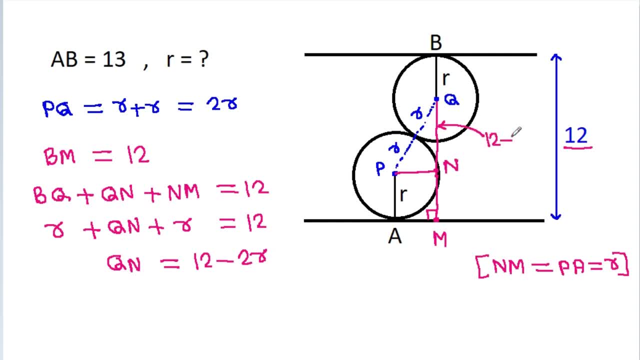 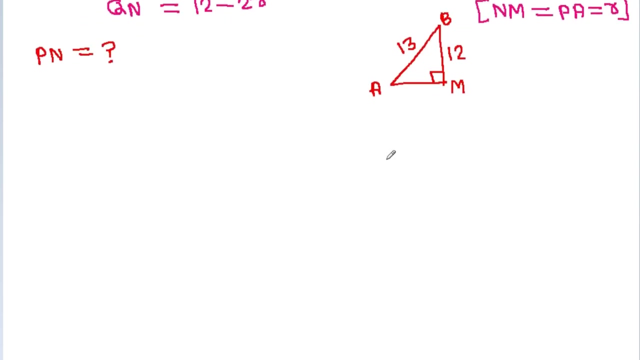 QN is 2N minus 2R, And can we find PN? What will be PN Here in triangle ABM? this angle is 90 degree, BM is 2N And AB is 13.. And by Pythagoras theorem. 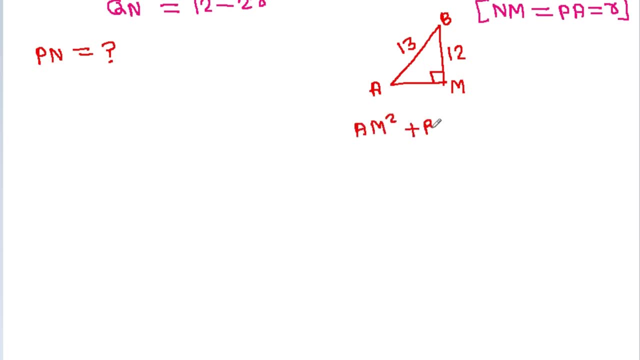 AM squared plus BM squared will be equal to AB squared, And AM squared plus BM is 2N squared will be equal to AB is 13 squared And AM squared plus 144 is equal to 169.. So AM squared will be equal to 169 minus 144,. 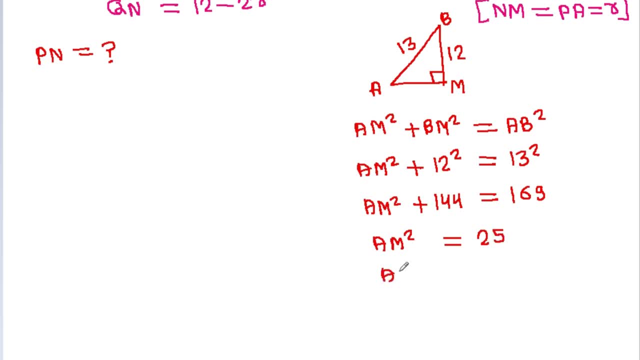 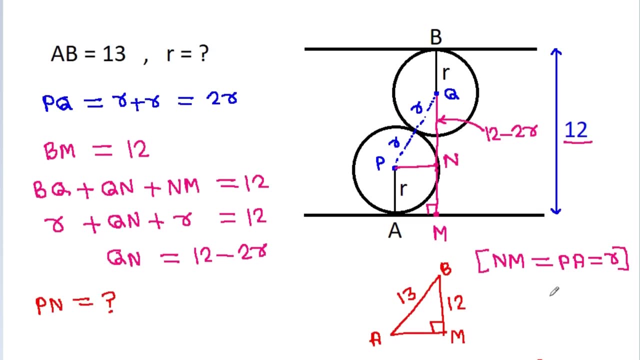 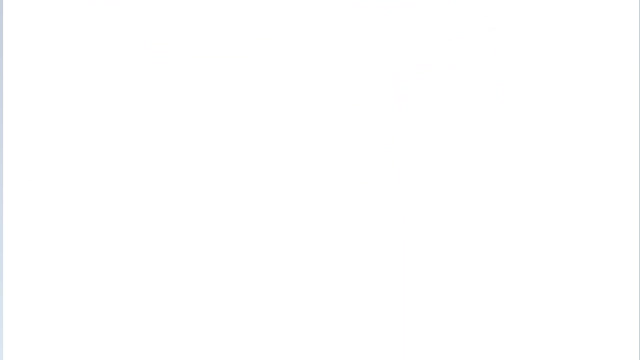 will be 25.. So AM will be 5. And AM will be equal to PN. that will be 5.. PN is equal to 5., PN is 5. And this angle will be 90 degree. So in triangle, 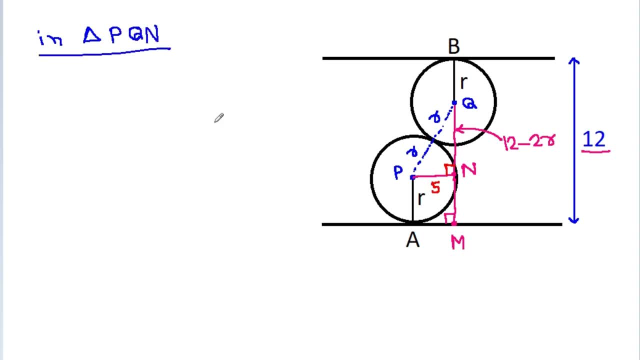 PQN. this angle is 90 degree. PN is 5.. QN is 2N minus 2R And PQ is 2R. So by Pythagoras theorem, PN squared plus QN squared will be equal to PQ squared.